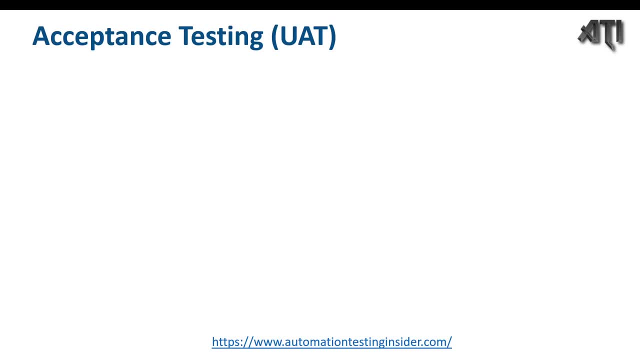 acceptance testing or UAT testing, and why do we need UAT testing and how do you perform this UAT testing? So let's get started. So take an example: guys, we are working for this company, So this is our software development company. We are working for a software development company and this is. 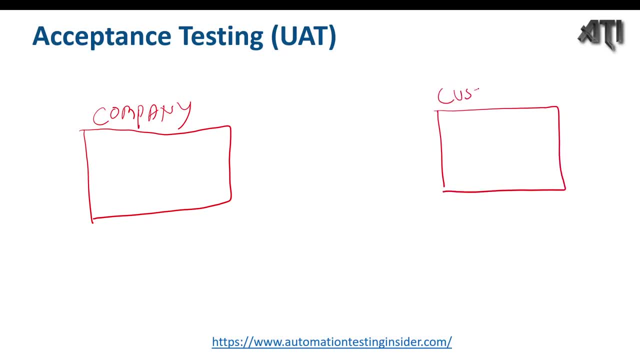 the customer which we are dealing with Now. this customer wants to have a software and they want to get build a software from our company. So they requested our company to build a software for their clients. So what they will do? they have given their requirements in the form. 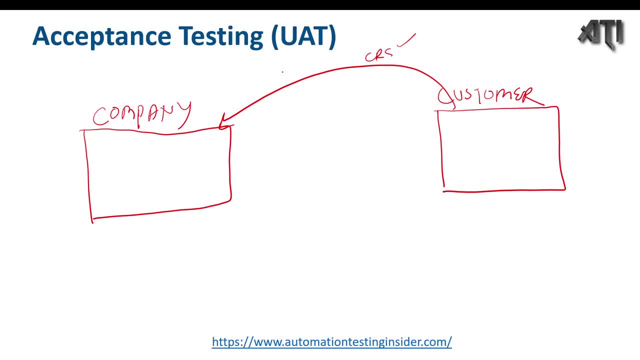 of customer requirement specification. Now what our company will do. our BA's business analyst work with their requirements, work with client or customer and get the requirement in the form of CRS, and we are- we are BA- will convert them into different documents for our company's understanding, like we have. 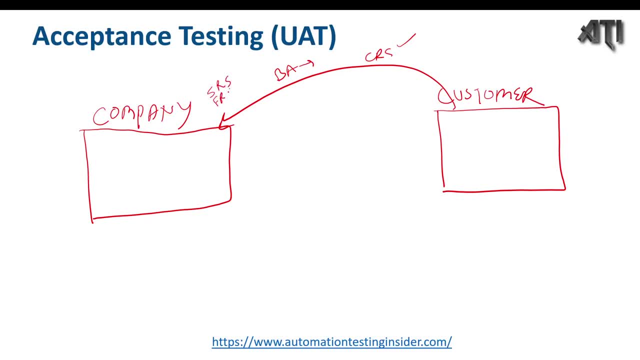 software requirement in specification. we have functional requirement specification or we have business requirement document. This is just for our understanding. BA will convert them into different documents, which we have already spoken about at the time of software development life cycle. Now what our company will do: now we got the requirement and we'll develop a software. 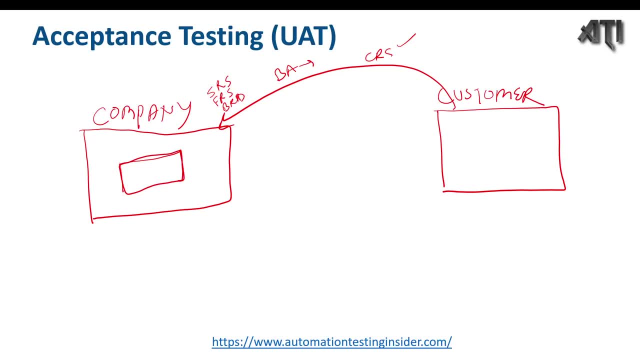 We'll develop a software or application for customer and once we have to follow the software development lifecycle correct, we have followed the software development lifecycle to build this software Like. we have requirement analysis, we have feasibility study, we have design coding. Now, when we talk about testing, we have performed different testing. we have done. 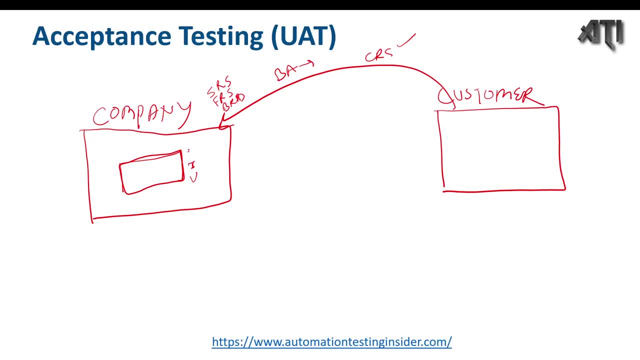 unit testing, we have integration testing, we have system testing. Now we need to perform the highest level of testing, which is acceptance testing. so how do we do this acceptance testing and why do we need acceptance testing? so what happens is, whenever we build a software, 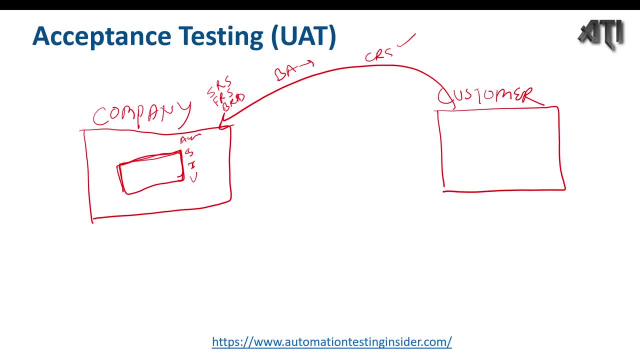 customer wants to have a final look of the software, like how the functionality is, how the workflow is, how the interface is and how the feature. what are the features they have included? they have included as per our requirement or not? so this is what the customer wants to do, the uat. so this is one of the reasons they, because they are paying. uh, they are paying for. 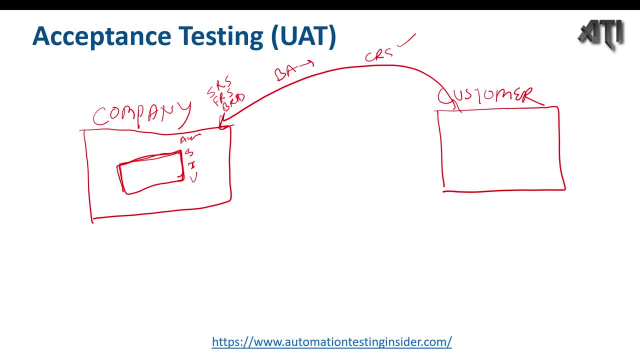 this, uh, software right, they are paying to our company to have the software, to get the software. so they want to have a final look of the software. they want to review it. so that is the reason they want to do the uat testing. that is, user acceptance. so based on that, they will accept the software. 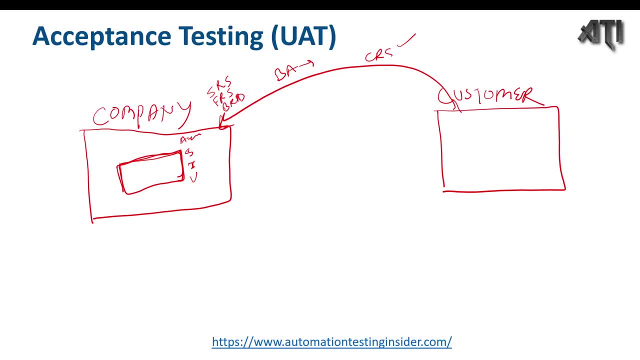 they will accept the application now. user acceptance, another reason could be. so, what ever documents we have written over here, we have gathered the requirement from the customer that might be misunderstood by our developer while developing the software, software by our development development team and testing team while developing the software and testing the 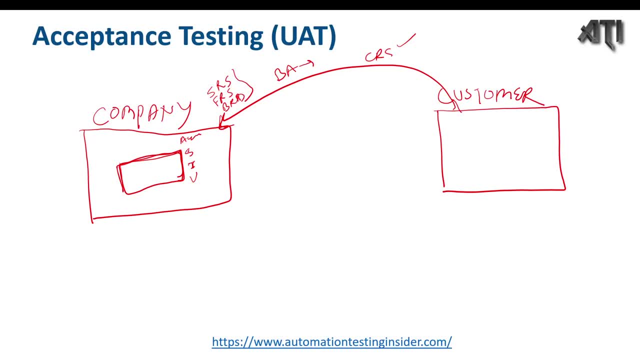 software. so that is that could be another. another reason: customer wants to review the software whether they have captured all the requirement or not. they have implemented all those requirements as per our expectations or not, whether the design is uh, design, uh, whatever they have designed in the application. 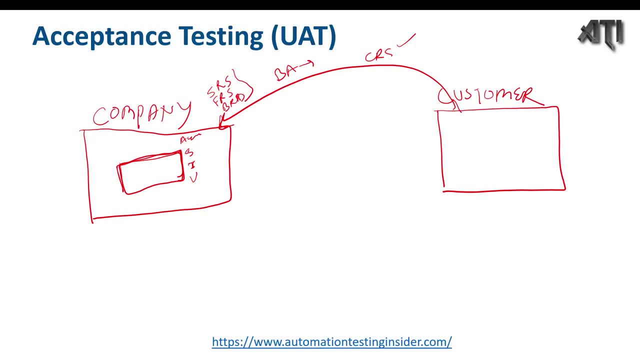 uh, that fulfill our expectations or not. that is the reason customer wants to do the uat testing. so in most of the companies, guys, uh, we have pre-uat and post-uat, and in some companies we do only uat testing, so pre-uat. so here we have pre-uat and this is also called alpha testing. 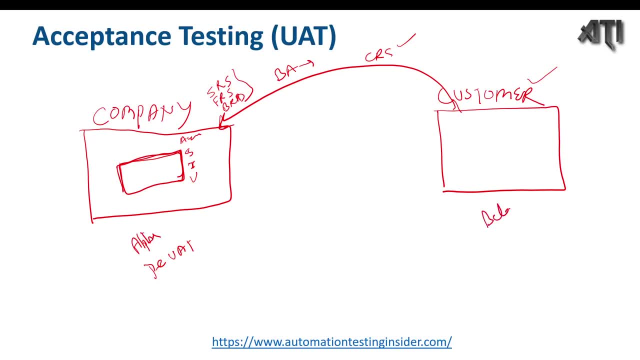 alpha and at customer end we do beta testing and this is called post uat- post uat. so now we'll do the pre-uat testing. we'll create test plan, priority test plan, scenarios and test cases and with our testers and bas involved in this priority test, and we'll do the pre-uat test at our end- alpha or alpha testing at. 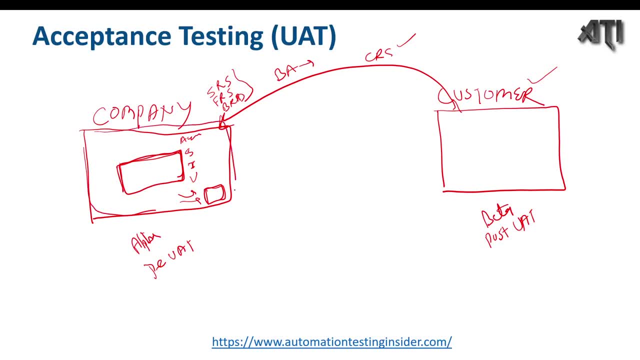 developers and this is development company guys. so our in testing environment will do the pre-uat testing now. if everything goes well, then we pass the priority test. otherwise, if we get any defect, then we'll get it fixed by the development team and we'll release the software to the. 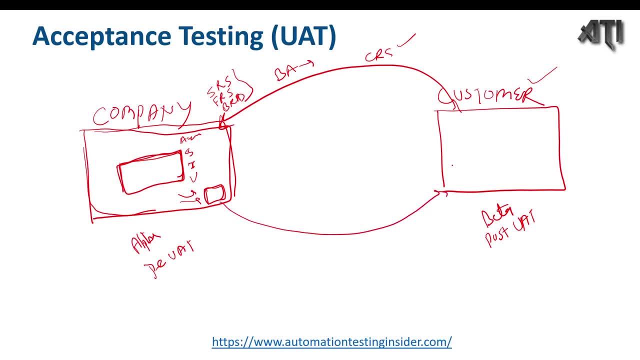 customer for beta testing or post uat testing. now they will perform at their end. this is real, a real time environment. guys raised real time environment or staging environment, just like production. so this is production environment. so it will just, it will be just like production environment. so they will execute some real time scenarios. they have their own testing team there. 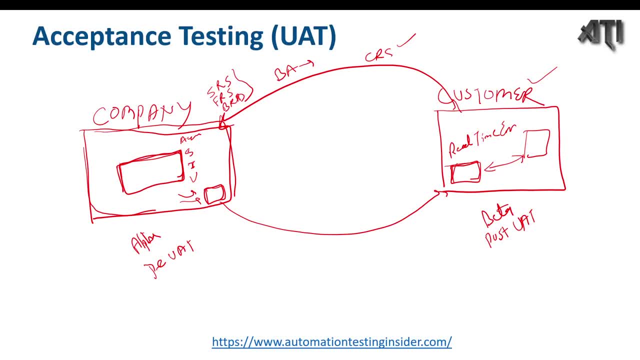 including bas, so they will perform the post uat testing. so they have set of uat test cases and they will execute those test cases. now if they are not happy with some of the requirements which we have developed, so they will revert it back. or if they get any uat defects, so they will revert it back to our development team. now we'll 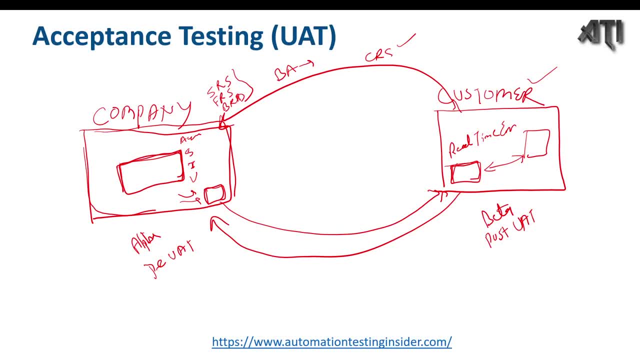 redevelop those functionalities or requirements from the customer or suppose they have missed some requirements from while giving the crs at the time of initial requirement, given giving the while giving the at the time of initial requirement. if they missed some requirements, so they will add while doing the uat and they will revert it to the development. 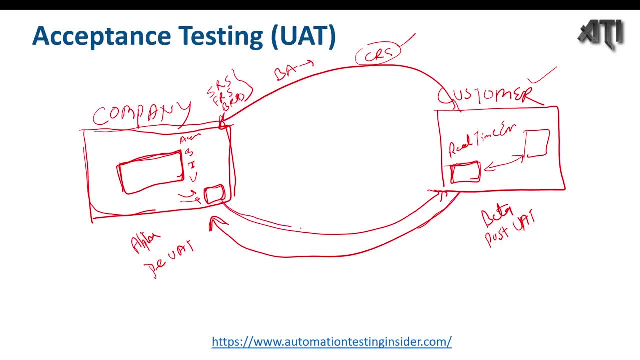 team now we'll redevelop all those requirements and we'll revert it back to the customer again. again, they will do. they will execute their uh post uat test cases or beta level test testing. they will perform now. if everything goes well, they will release the software into production. 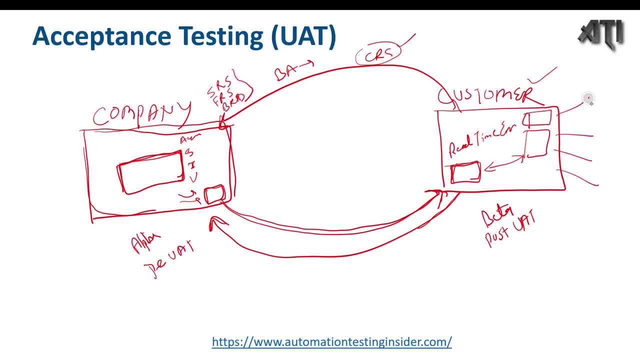 with and they will release the software to their customer, their own clients. so this is how it is uh happening, guys: acceptance testing or uat testing. so, as i have told, like some companies, they are following pre-uat and post-uat, which is called alpha testing and beta testing. 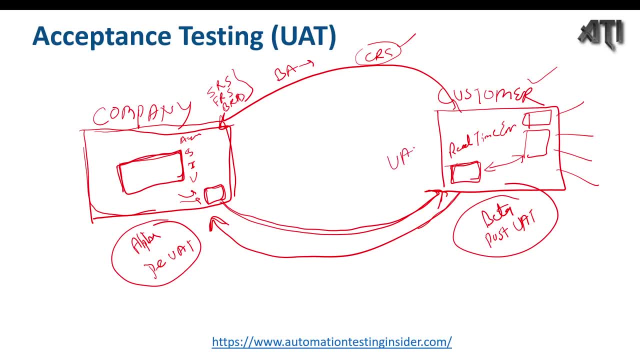 and in some companies we used to do only uat at at customer end. so this is all about acceptance testing, guys. now let's talk about uh, like theoretical stuff, and what is alpha testing exactly and what are the different advantages of alpha and beta testing. so let's start with the 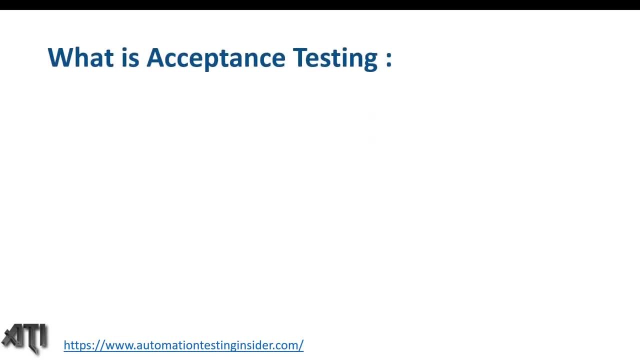 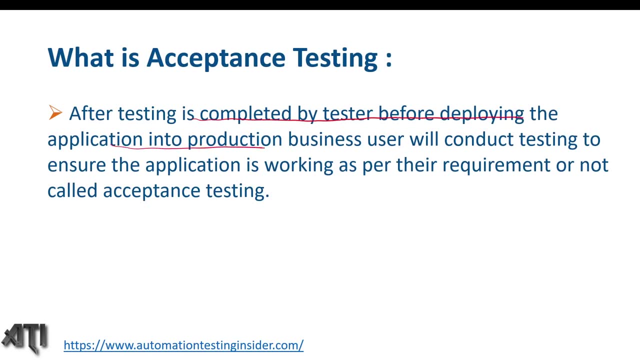 let's move on to the next slide. so after testing is completely completed by tester, before deploying the application into production, business user will conduct testing to ensure the application is working as per their requirement or not, called acceptance testing, which we have discussed. this is the type of testing done by. 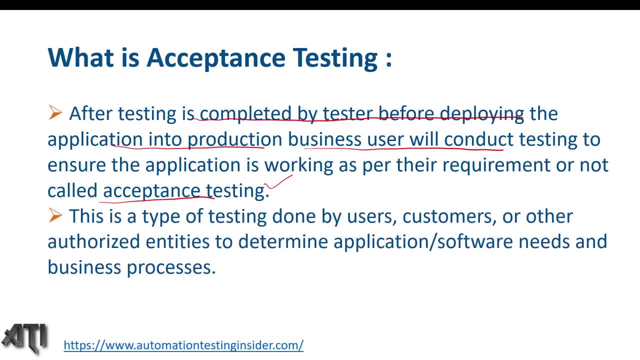 users, customers or other authorized entities to determine application software needs and business. so this is done at our end, which is developers and is which is called alpha testing. another way to do uat is if they release their software to their own customers so we can do the uat at their 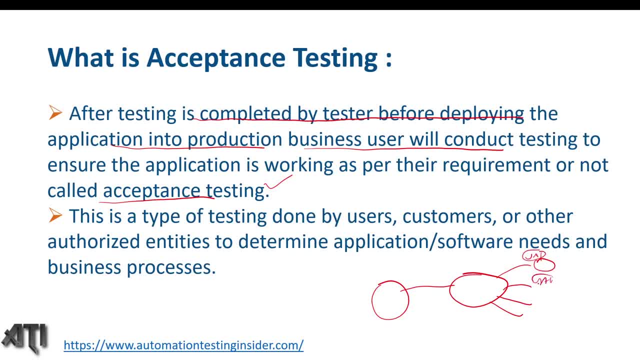 end as well. they will perform the uat at their end as well. so that is another way to do the uat testing, software testing, where a system is tested for acceptability, so whether to accept that software or not, so that is evaluate using this uat testing. 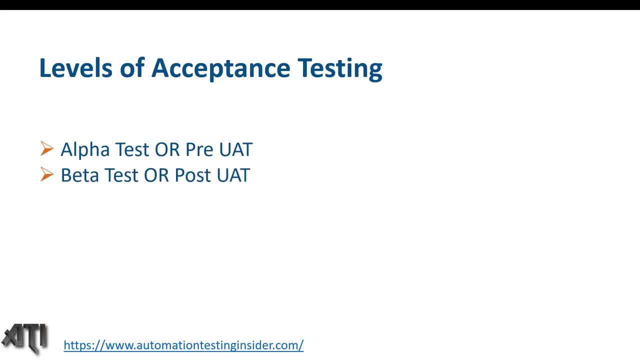 so what are the different levels of acceptance testing, guys? so we have discussed, we have two levels: alpha test or pre-uat, beta test or post-uat. so here you can see alpha testing and beta testing. advantages of acceptance testing: so reduces the risk of defects being identified in production. 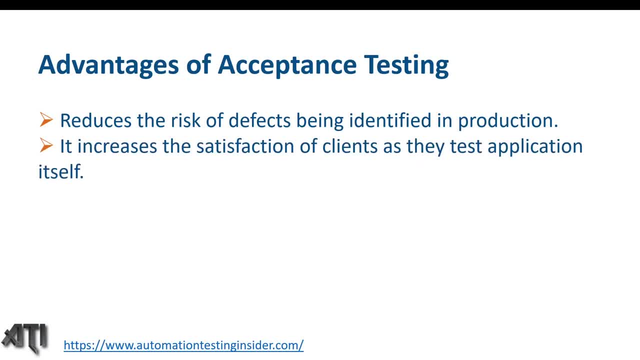 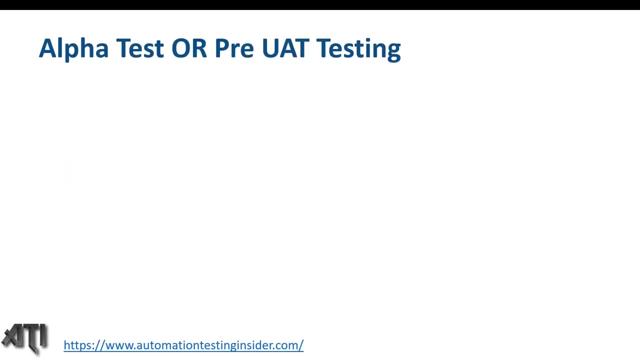 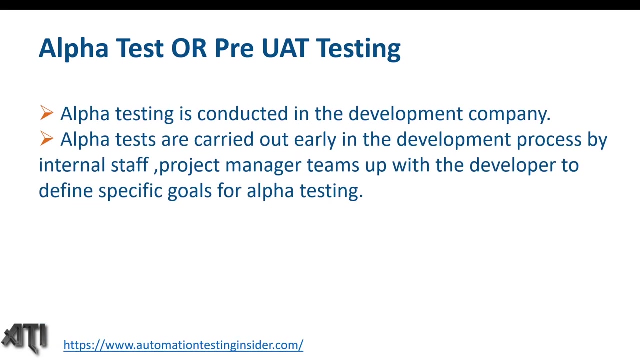 it increases the satisfaction of clients as the test application itself, increasing software robustness and usability and increase end user happiness. so these are the different advantages of doing acceptance testing. guys, let's talk about alpha test. alpha testing is conducted in the development company which we have already spoken about. alpha tests are carried out early in. 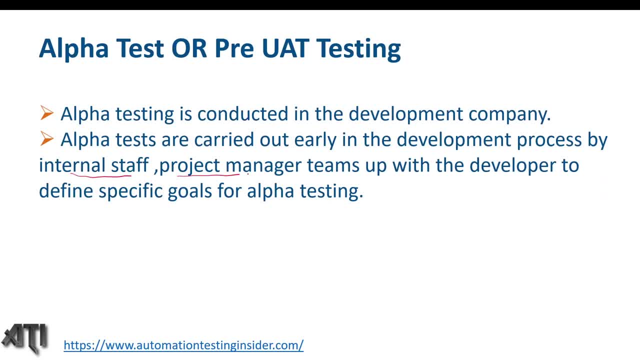 the development process by internal staff. project manager teams up with the developer to define a specific goal for alpha testing. so we have already spoken about alpha testing. we have already spoken. testing is conducted in test environment, so this is what we have spoken about. testing is done by testers and quality analyst, so quality analyst is nothing but the business.